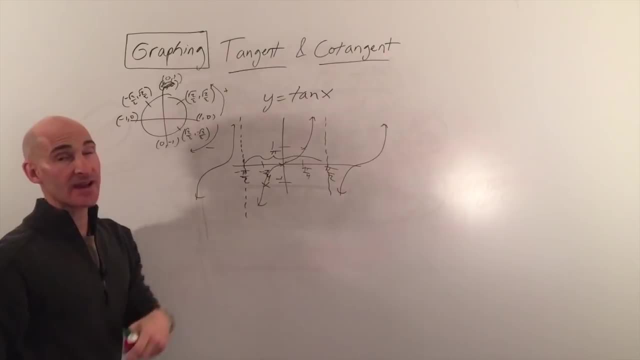 one period is pi. So remember, for sine and cosine the period is 2 pi. normally For tangent and cotangent it completes one cycle and one pi. Okay, so now what we're going to do is we're going to look at what happens if you stretch this graph, compress this graph and so on. But before we do, 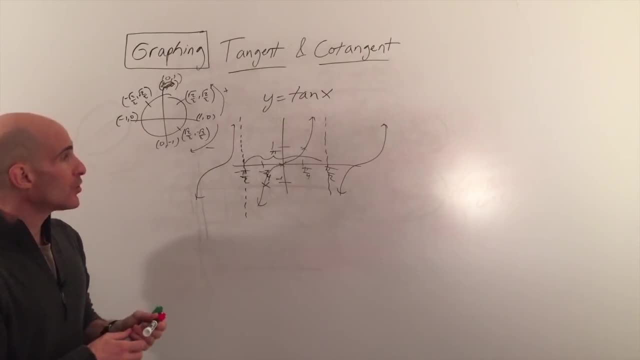 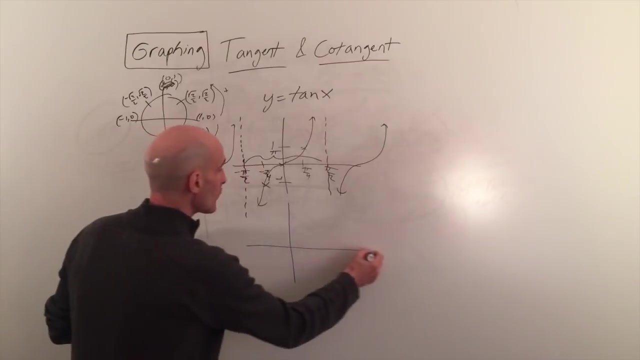 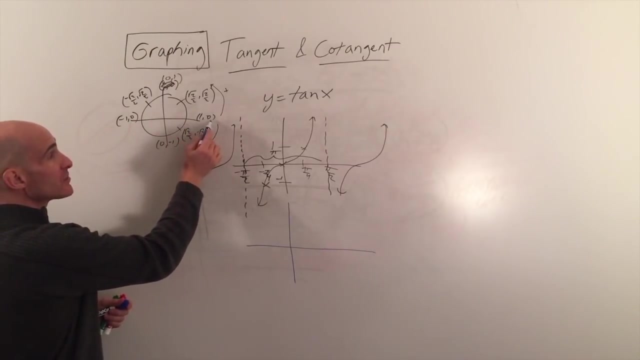 that. let's take a look at cotangent. So we've got the unit circle right here. So cotangent- I'll put it right underneath tangent so you can kind of compare and contrast. So for cotangent we're going to look at the points from 0 to 180, 0 to pi. So cotangent is x over y, So 1 over 0. 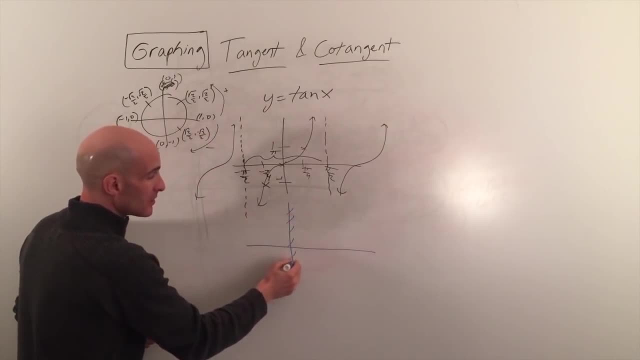 that's undefined. You can't divide by 0, so we get a vertical asymptote: At pi over 4, x over y is 1, because anything divided by itself is going to give you 1.. At pi over 2, x over y, 0 over 1 is 0.. At 3: pi over 4. 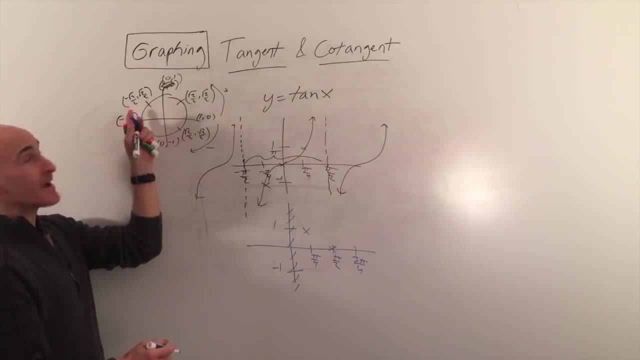 x divided by y negative square root, 2 over 2 over positive square root, 2 over 2 is negative 1.. And then if we go over to pi x over y negative, 1 over 0 is undefined. We get another vertical asymptote. 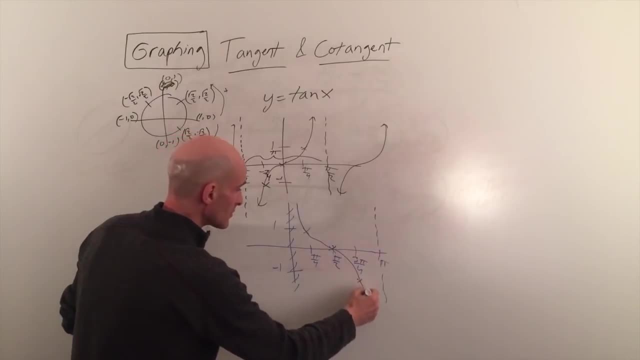 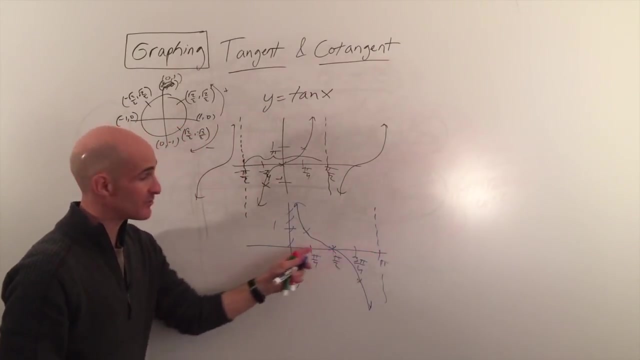 So for cotangent the graph looks like that And again it repeats: just like tangent. Okay, every pi, So that's period is pi. Now what some students remember is that tangent is going up to the right, Cotangent is going down to the right Tangent half. 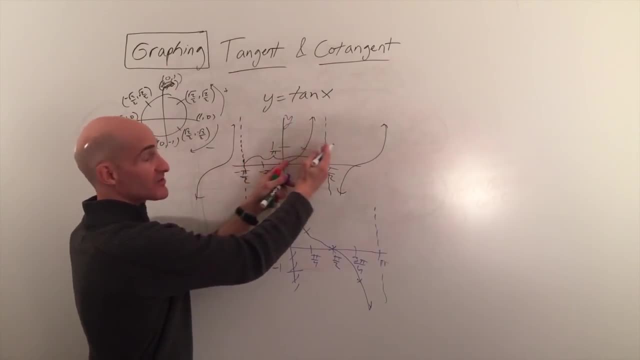 the graph is to the left of the y-axis, okay, half to the right, Whereas for cotangent, the whole graph is to the to the right of the y-axis here. Okay, so kind of notice the difference. So tangent, half is on the left, half is on the right side of the y-axis. Cotangent, the whole graph is to the right. 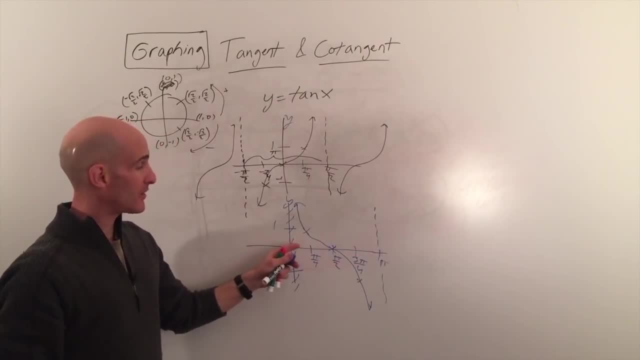 of the y-axis. They both have a period of pi, okay, and you can divide it up into four. So you can divide it up into four pieces, like we did here. These are the basic parent graphs, Okay, so what we're going to do next is we're going to look at the stretching and the compressing and the 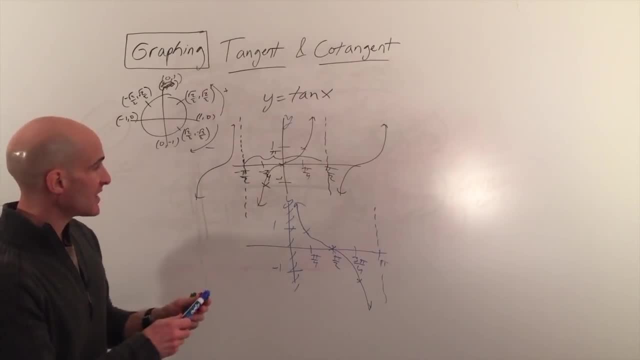 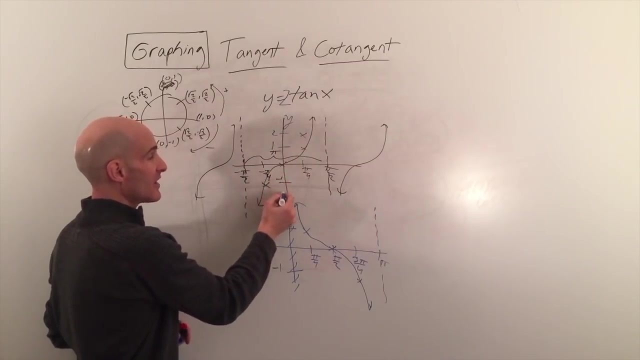 shifting, just like we did with sine and cosine. So let's just take a look. Say I want to graph: y equals 2 tangent of x. What do you think the 2 does to the graph? That's right, it stretches it. So instead of being here at 1, you're going to be up here at 2 now, Instead of being here at negative. 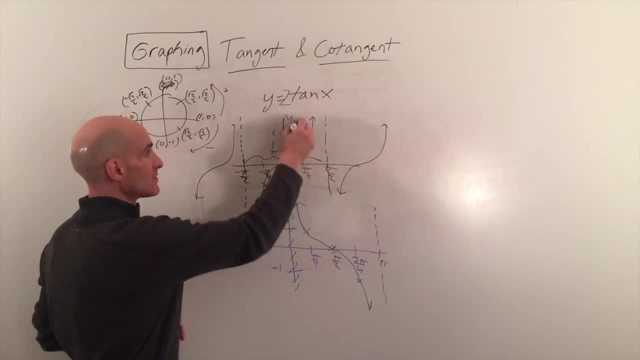 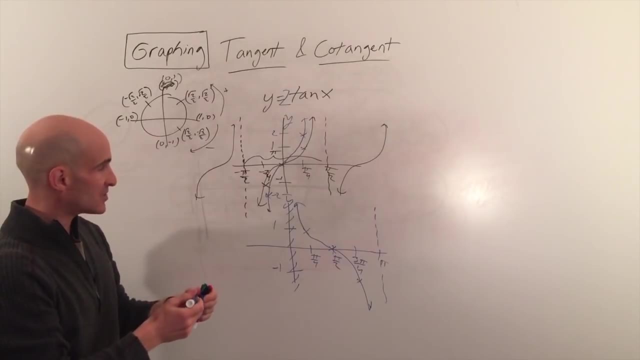 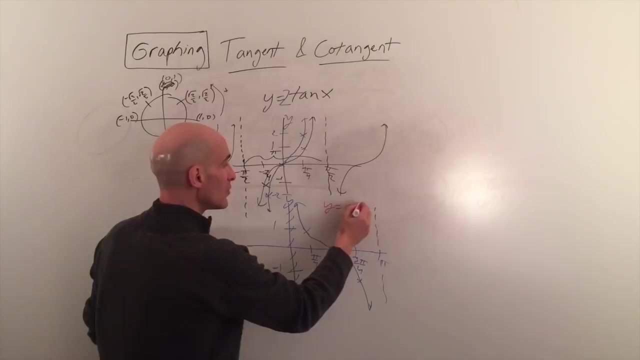 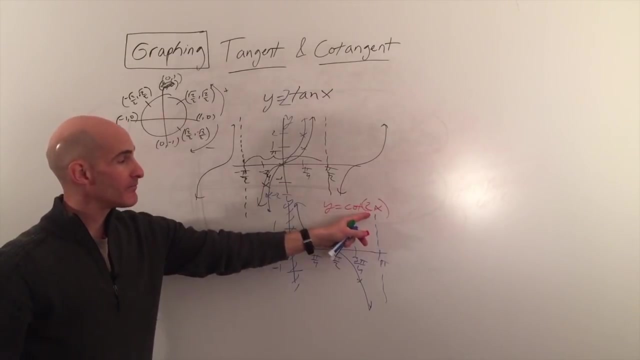 this is a vertical stretch, So it's like you're pulling on it. Okay, stretching it this way, Okay, it's the same thing for these. Okay, now if we look at cotangent, let's say, for cotangent, we want a graph. y equals cotangent of 2x. Okay, what do you think the 2 does to the graph? Well, we can use. 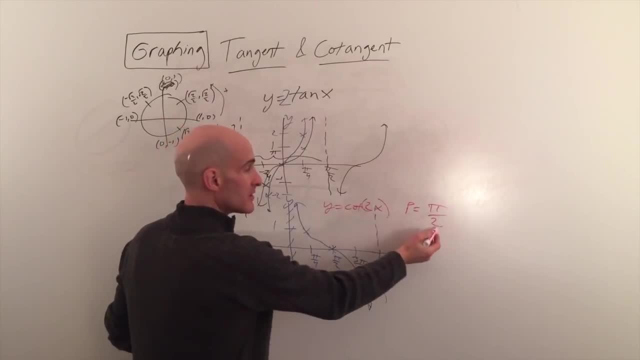 this, Okay. so what we're going to do next is we're going to divide the x values by 2.. Okay, so what that means is completing one cycle in pi over 2.. So what it's going to do is it's going to compress. 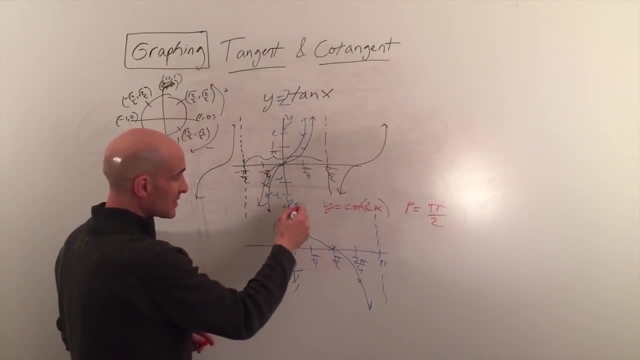 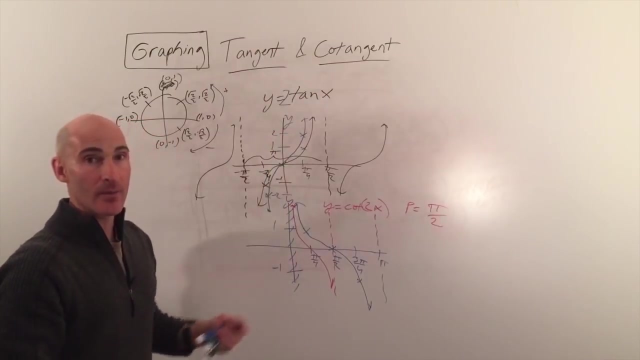 this. It's actually going to divide the x values by 2. It's going to complete one cycle like this: now It's compressing it, Okay, and then you can shift it to the left and right, up and down. So I'm going to erase this. 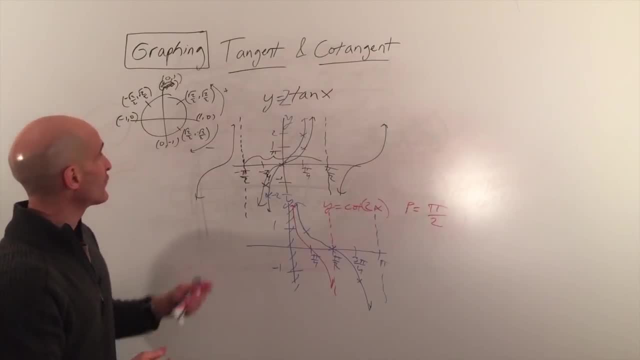 Real quick and we're going to take a look at some more difficult problems. But if you forget, just go back to the unit circle. Tangents y over x, from negative 90 to positive 90.. Cotangent from 0 to pi or 0 to 180.. That's x over y for cotangent And that's how you can get the parent graphs. and 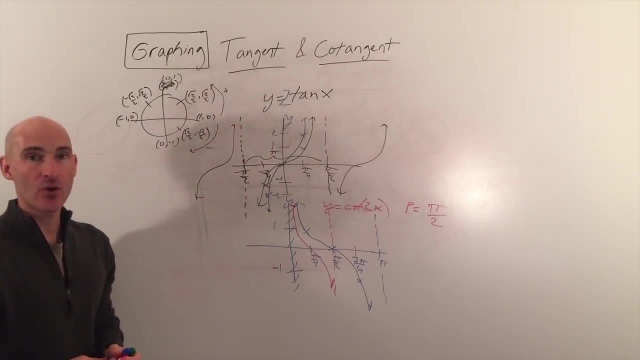 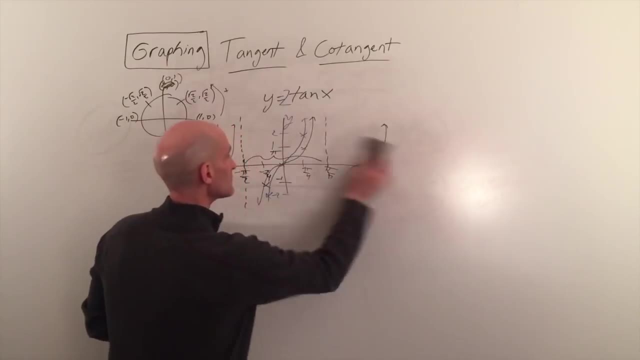 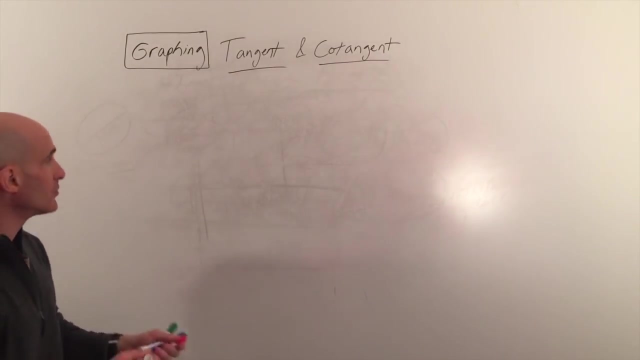 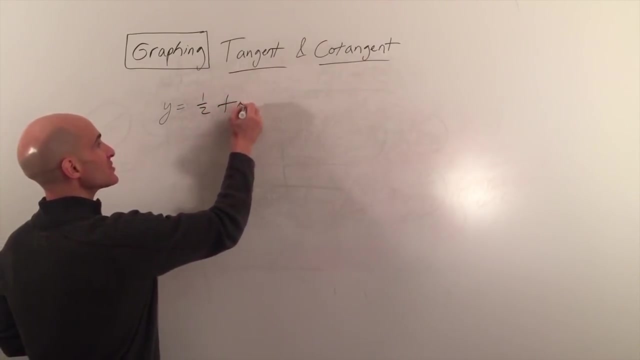 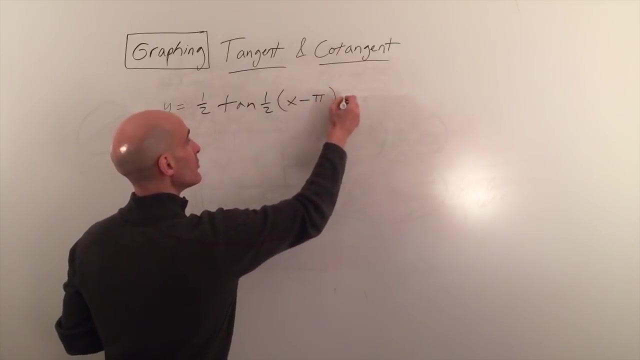 then you can stretch them, compress them, shift them and so on. Let's look at some more difficult problems and you'll see what I mean. Okay, here's a good one. right here, Let's do: y equals one half tangent one half x minus pi plus 2.. Okay, what I would do, just like we did for sine. 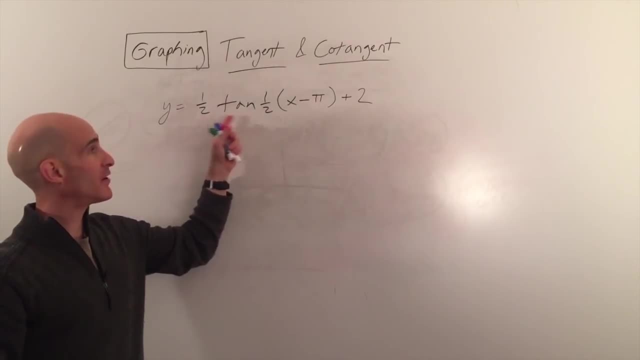 and cosines. I would graph the parent function using the amplitude, the a value and the b value which affects the period. Then we can pick up the graph and shift it Right. pi, Remember, this one has the opposite effect. This one has the same effect on the graph: Plus 2 is 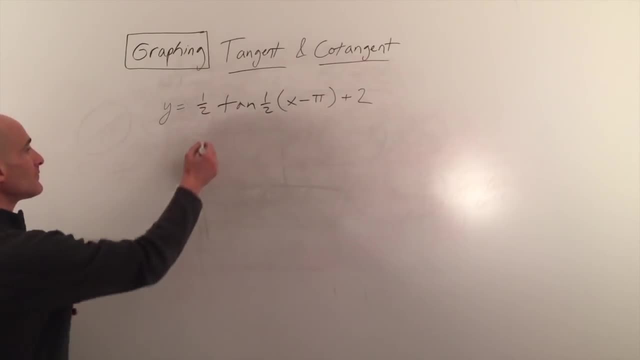 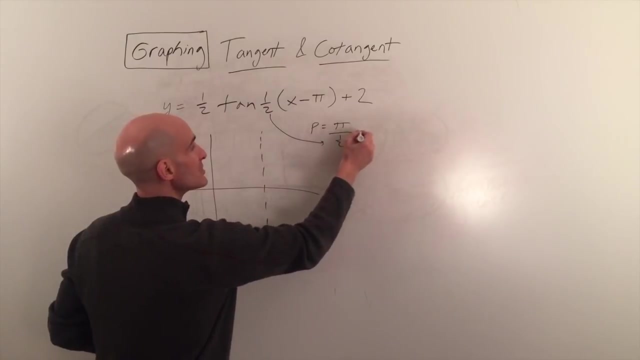 actually up 2.. So let's start by graphing this one here. Now I'm just going to start by graphing the asymptotes. I'm going to take the period which is normally pi for tangent and cotangent. I'm going to divide it by one half, which gives you a period of 2 pi. Because remember, when you divide, 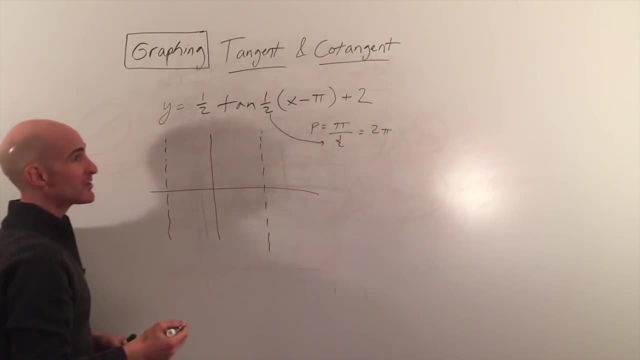 by a fraction. it's like multiplying by the reciprocal, So that's like multiplying by 2.. That's 2 pi. But what I'm going to do- and this is what some students get a little confused- by half's on the right side of the y-axis, half's on the left, I'm going to take this 2 pi. I'm. 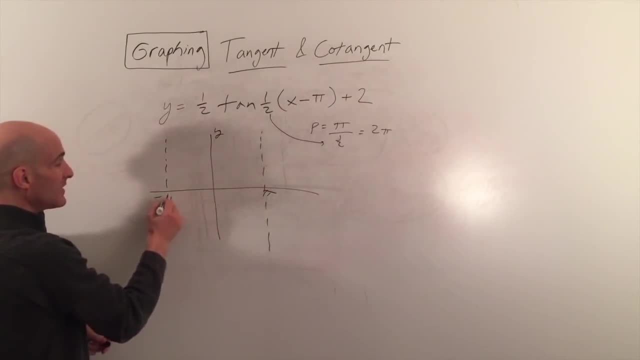 going to divide it in half. So this is actually pi here and negative pi, giving you a period of 2 pi. I'm going to divide it in half again. These are like our midway points: Pi over 2 and negative pi over 2.. And then the amplitude is a half. So we're going to go up here to a half. 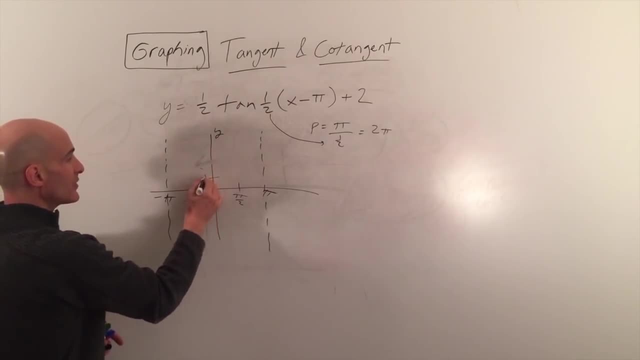 And let's- let me erase this a little bit- Let's put a half over here And negative a half down here, Okay, and so our graph is going to look like this: Okay, that's our parent graph. Okay, but then what we're going to do is we're going to shift it, right? 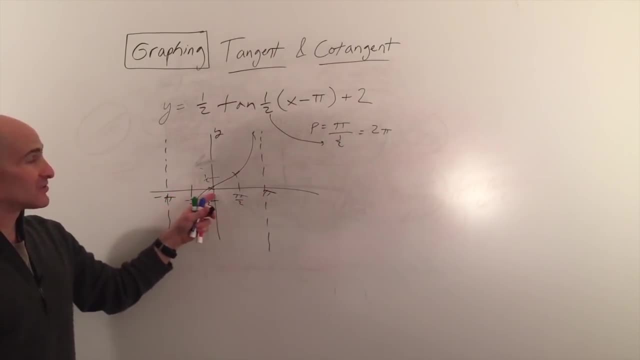 pi and up two. Now, on our scale, pi is actually two steps. So everything is going to shift two steps to the right and up two steps. Okay, so what we have to do here is we're going to take each of these asymptotes, We're going to shift them right two. So now your asymptote is: 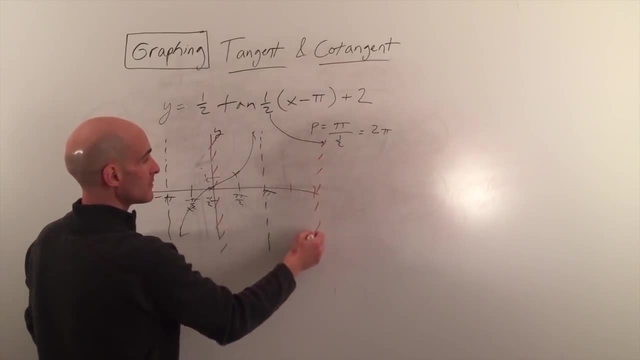 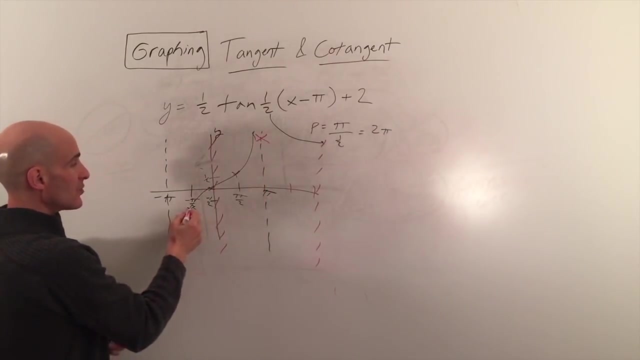 right there. This one's going to go right here, This point's going to go here and up two. So I'm just going to estimate for this. This is going to go right. two, Okay, and up two. I'm just going to. 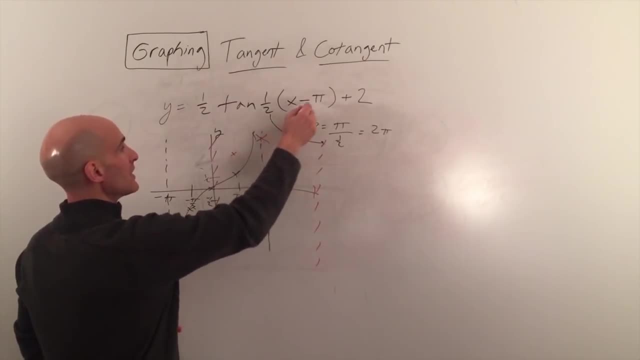 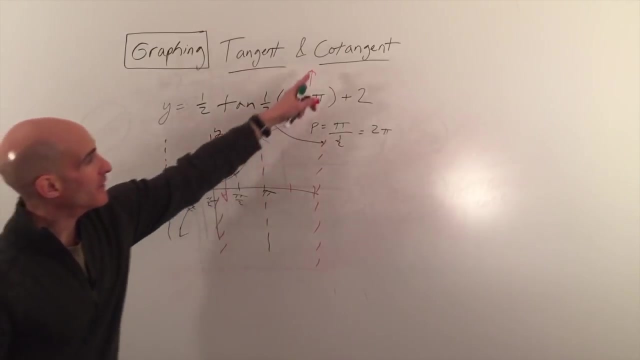 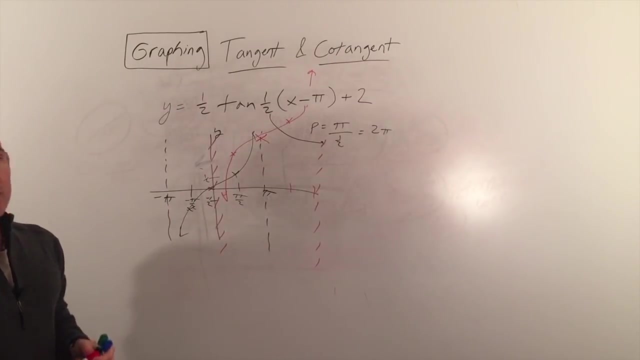 estimate for that. And then this one's going to go right two and up two, And so our graph now looks like that. Okay, the red graph. So it shifted right two and up two based on the scale that we had. Okay, so that's tangent. Let's do a more challenging cotangent graph. 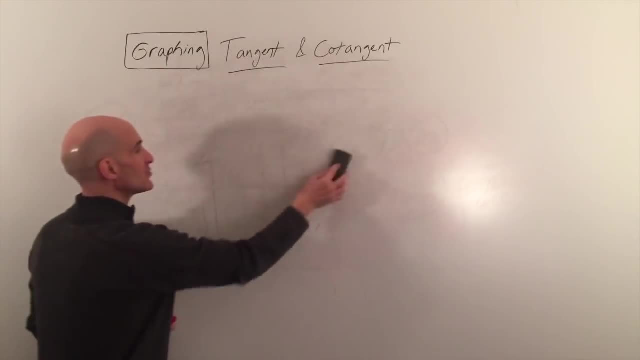 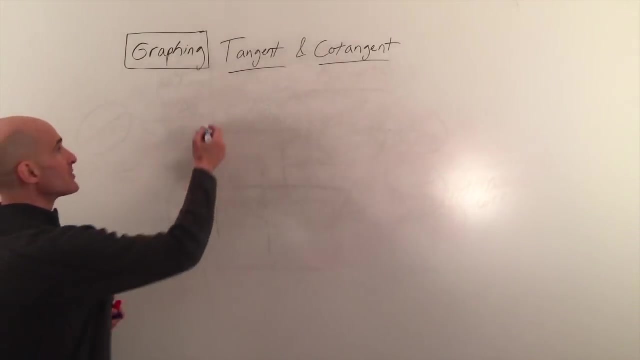 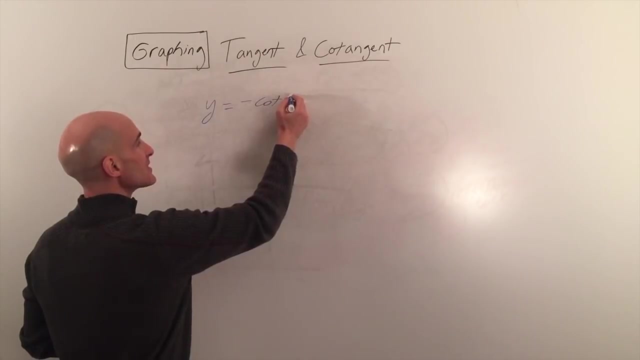 The key, I believe, is to do it in steps. You know, graph the amplitude and period in one step, Then you can graph the shifted graph in the second step. So let's graph this cotangent graph. Let's just say: we're going to graph: y equals negative cotangent. Let's just say: this is 2. 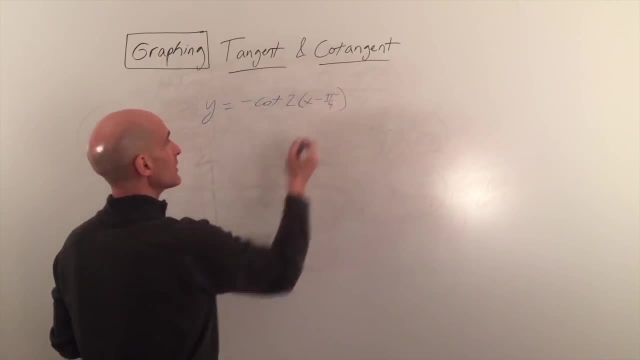 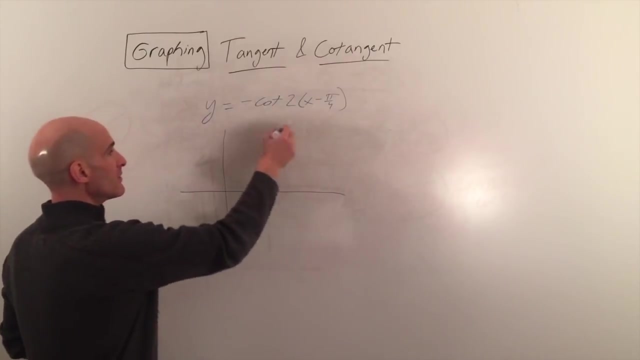 x minus pi over 4.. Okay, we'll just do this one a little bit more simple. So cotangent looks like this: Here's the y-axis. Here's the x-axis. It goes down to the right like that Gets to the. 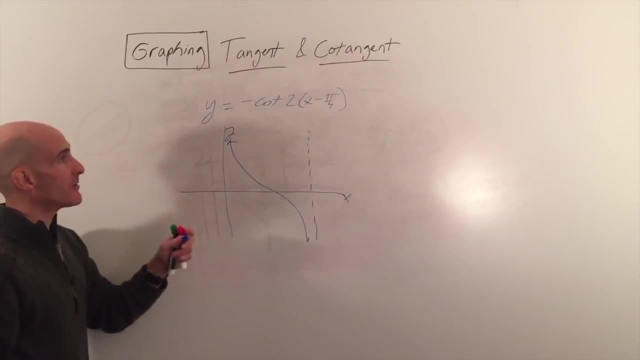 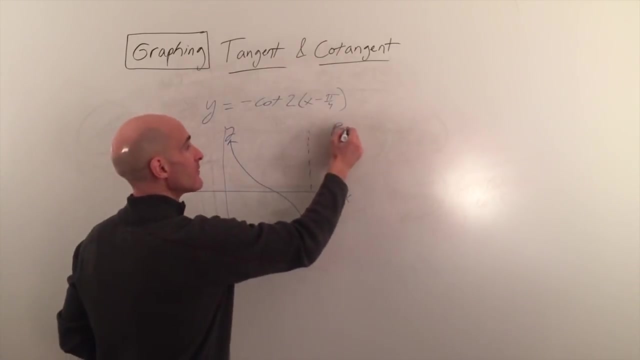 right of the y-axis, Whereas tangents half's on the left, half's on the right. The period is going to be 2 pi divided by two, I'm sorry, one pi Tangent, cotangent. the period is normally pi. 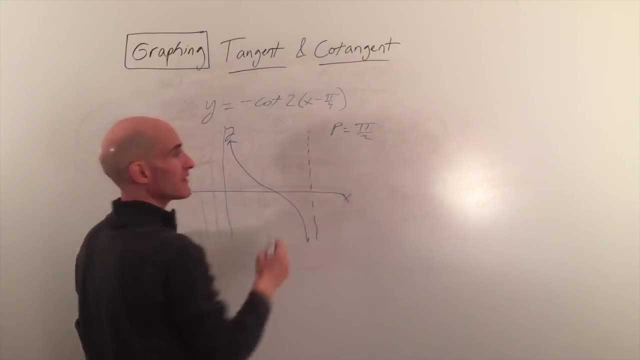 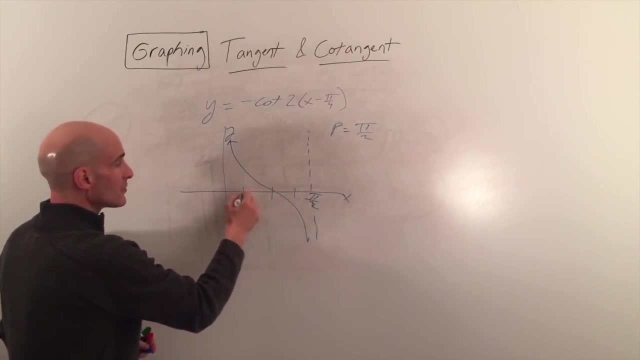 Sine and cosine, and period is 2 pi. So we take pi divided by 2.. Okay, so that means one period is going to be completed in pi over 2.. I'm going to divide this into 1,, 2,, 3,, 4 pieces. So this is pi over 4,, pi over 8, and 3 pi. 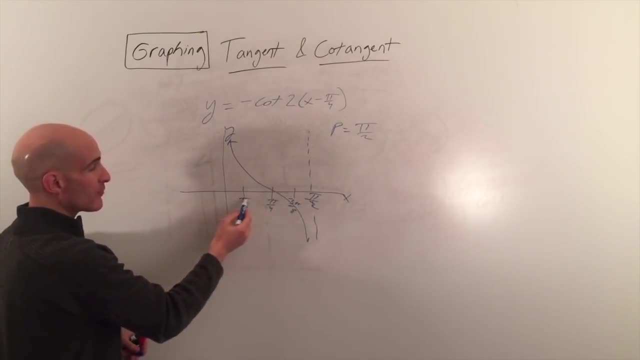 over 8.. Okay, so you could take pi over 2 divided by 4.. That's pi over 8.. And that's going to give us our scale. Now the negative. What do you think the negative does? The negative reflects it over. 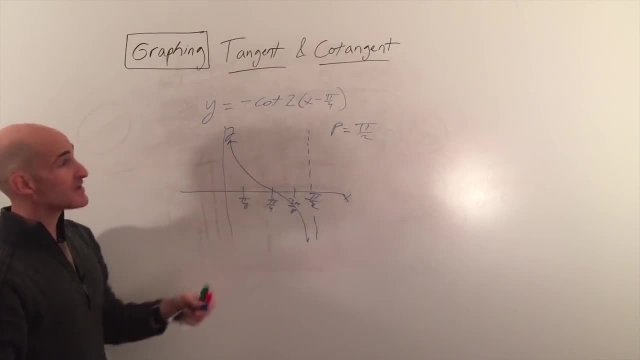 the x-axis It makes, the positive y-value is negative and the negative, 1, is positive. And what do you think the pi over 4 does? Shifts it. right, pi over 4.. So everything's going to shift, even these asymptotes. Okay, right, pi over 4.. Now, on our scale, that's going to be two units to the. 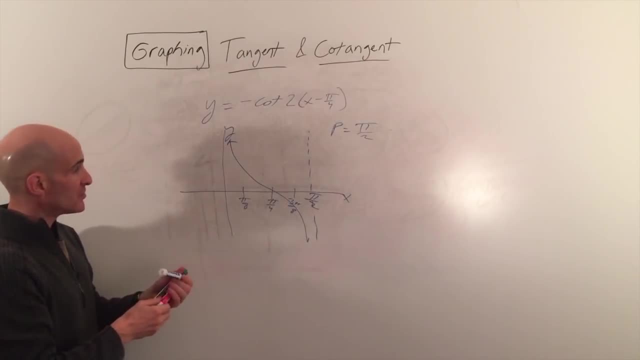 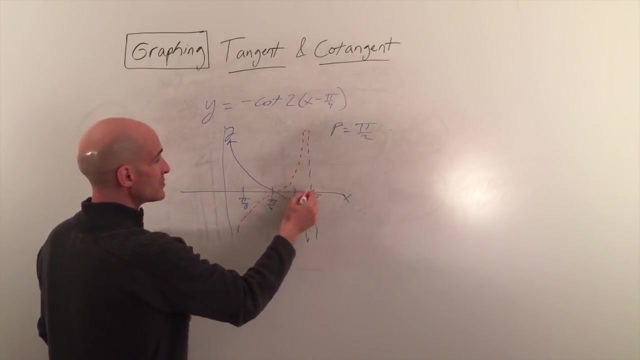 right, because we're counting by pi over 8.. Okay, so what I'm going to do is I'm just going to: first I'm going to reflect this, So the graph looks like this, Okay, and then it's going to shift right, pi over 4.. So these points are going to go: 1, 2, 1, 2,. 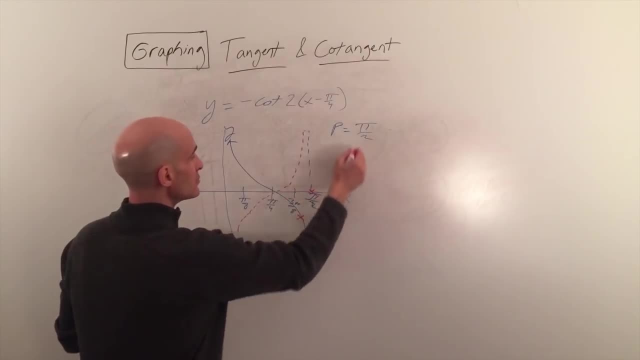 2.. And the asymptotes also are going to go 1, 2, and 1, 2.. So your graph now is going to look like like this: Okay, it's going up to the right because it was reflected over the x-axis by this negative here. 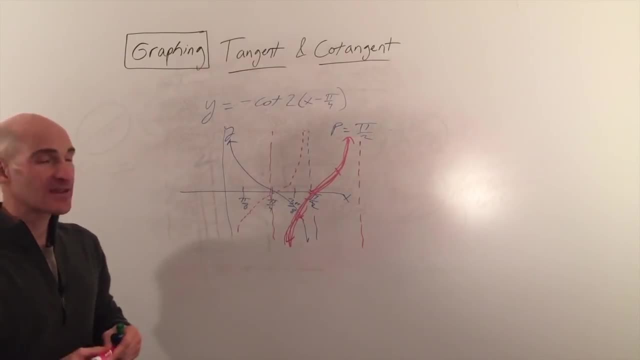 So that's cotangent. We talked about tangent And if you just go back to the parent function, like I said, do the a and the b first and then you can shift it second, The graph down. So that's tangent and cotangent. Take a look at the graphs I did on sine and 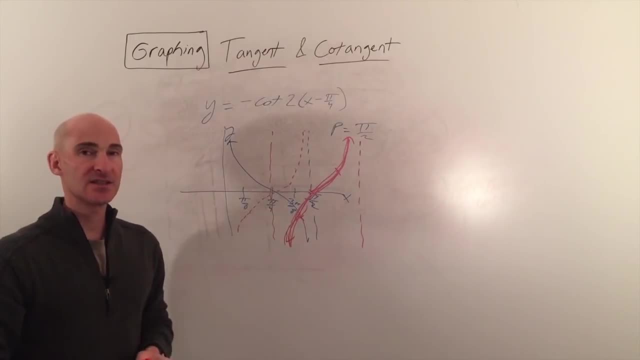 cosine for additional pointers And we'll take a look at secant and cosecant in the next video.